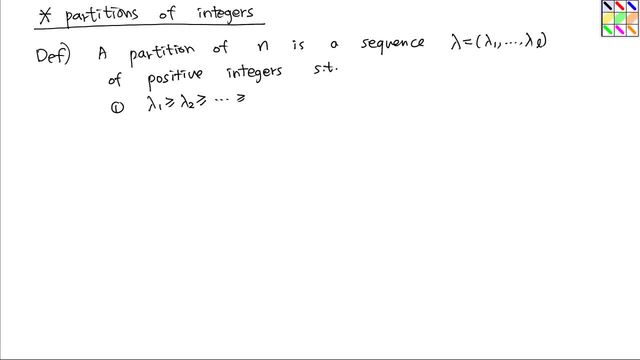 than or equal to lambda 2, greater than equal to lambda L. It's a weakly decreasing sequence, Decreasing. and second, their sum is equal to L, and so in this case we say that each lambda I is called a part, and the number of parts of lambda is denoted L of. 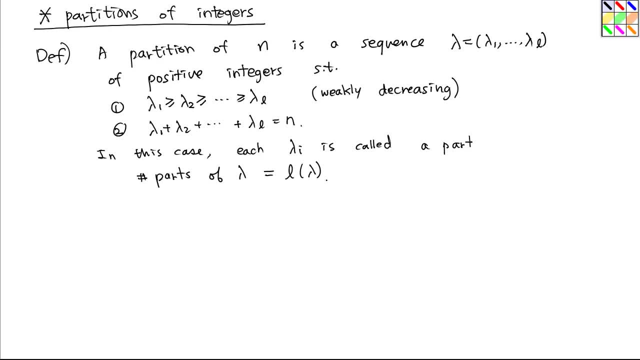 lambda It means the length is also called the length of lambda. So if there are L parts then the length is L. So we will rewrite: lambda is a partition in the in this notation or absolute value of n. They both mean that lambda is a partition of n. So an example: 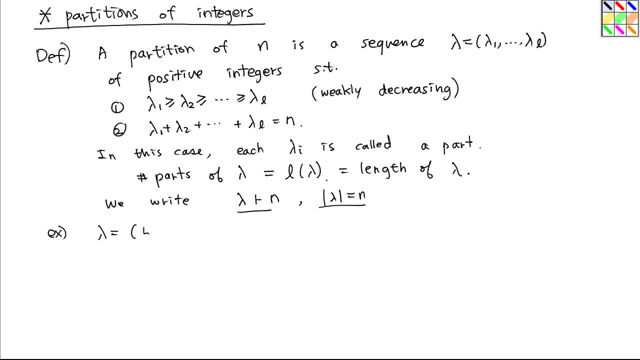 if lambda is the sequence 5 comma 3 comma 3 comma 2 comma 1, then this is a partition of lambda, Because integers are weakly decreasing and their sum is 14.. So in this case we're going to write: lambda is a partition 14.. This, or equivalently, lambda is a. 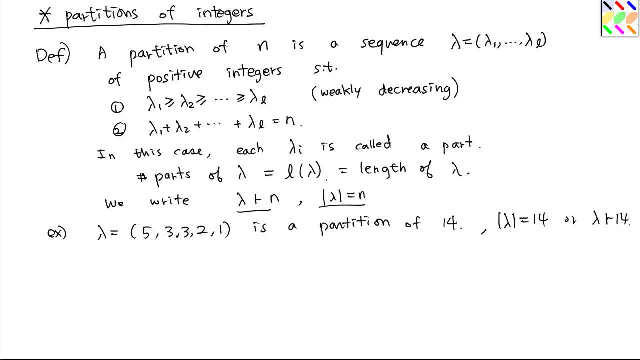 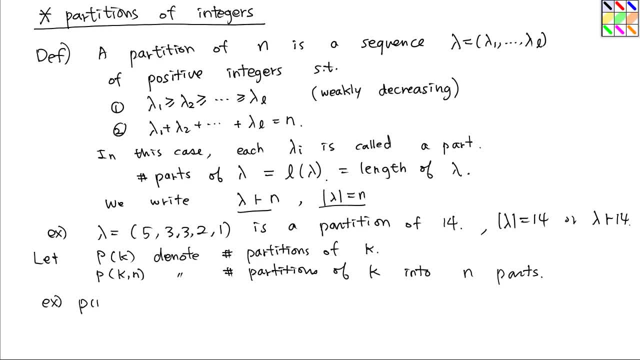 So, for example, p of 1 equals 1, because number of partitions of 1 is 1.. 1 is the only partition and p of 2, partition of 2, there are two, so it's going to be 2.. Number of partitions of 3.. 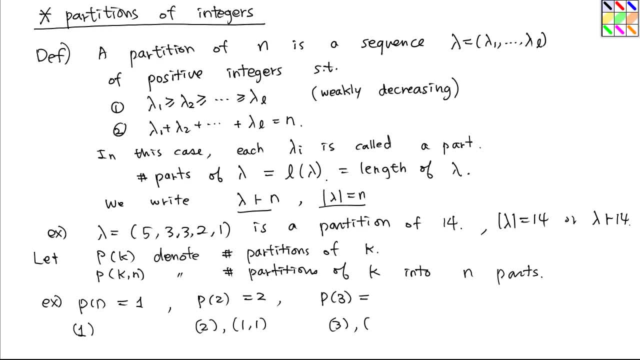 We have 3 and 2 comma, 1.. 1 comma, 1.. 1, 1, 1,, so it's 3.. And P of 4, partitions of 4, 4, 3, 1, 2, 2, 2, 1, 1, 1, 1, 1, 1, 1.. 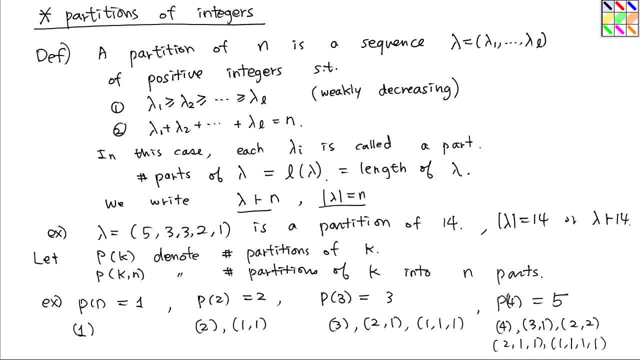 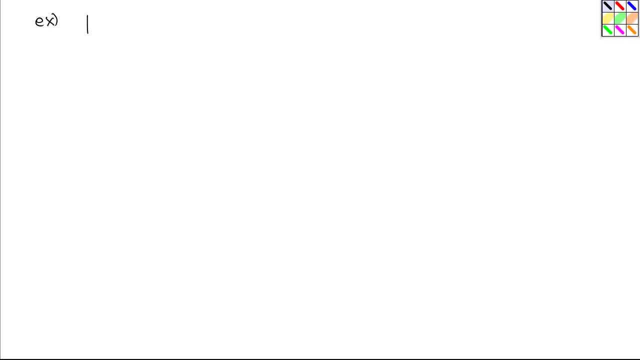 So there are 5 partitions of 4, so it looks like this. Next, and continuing the example P of 5, 2,, so 5,. in order to write 5 as a sum of 2 integers, you can write 4 and 1, or 3, 2.. 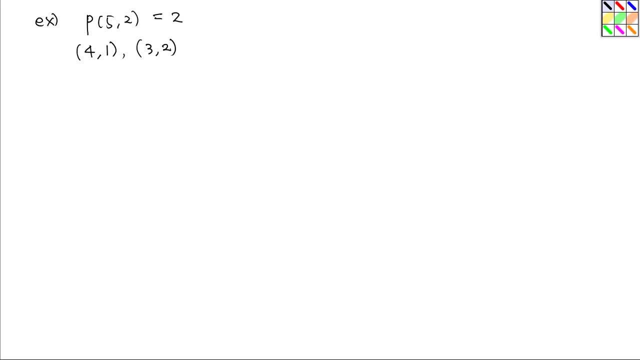 So there are only 2 decreasing sequences of length, 2 with sum equals 5.. So let's do one more example: P of 8, 3.. So 8 can be written as: let me write this: 8 as a sum of 3 integers. 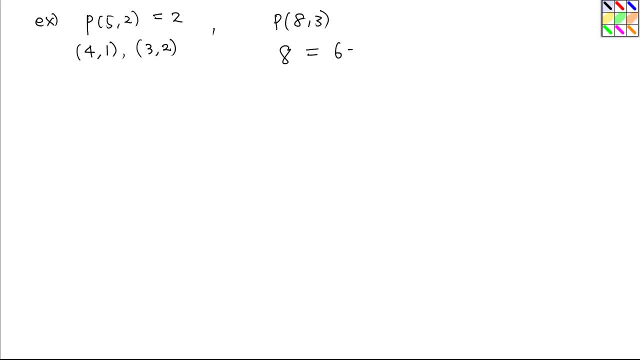 So it can be 6 plus 1 plus 1,, or 5 plus 2 plus 1,, or 4 plus 2 plus 2,, 4 plus 3 plus 1, or 3 plus 3 plus 2.. 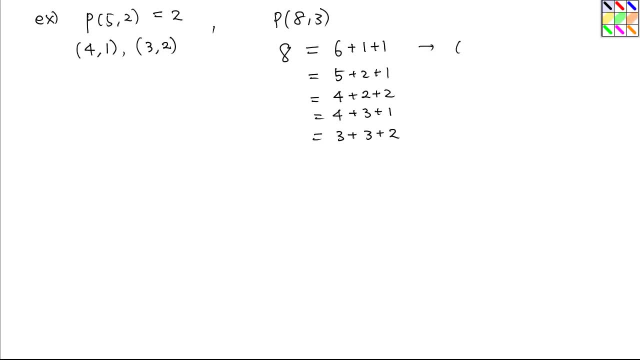 So this will give us this 6, partition: 6, 6, 6.. This will give us 5, 2, 1, 4, 2, 2, 4, 3, 1.. 2, 4, 3, 2, 4, 1, 2, 2, 1, 2.. 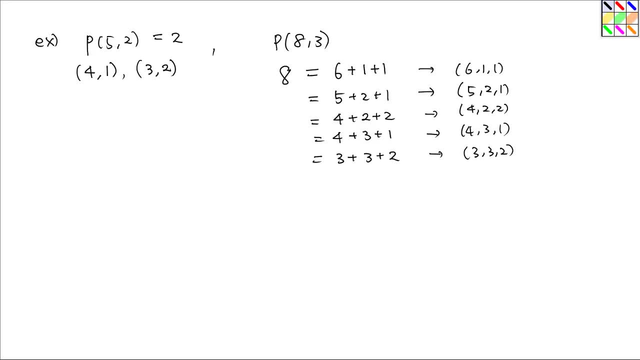 1, 2, 3, 2, 3, 1, 2, 2.. These are all the partitions of 8 into three parts, so it's going to be 5.. So, like I did here, you can think of this partition as a way of expressing this number. 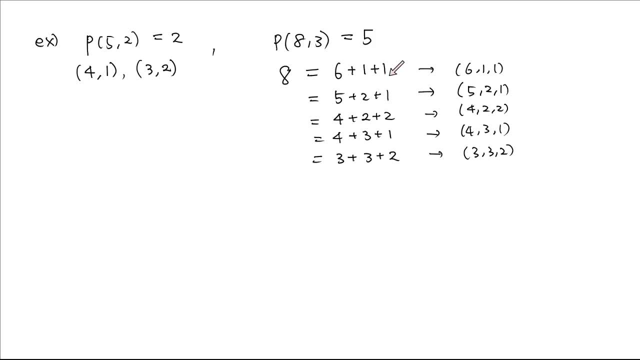 as a sum, but we always write the numbers in weakly decreasing order. Okay, And this definition of partition is very simple, but surprisingly, there are no formulas, no simple formulas for these numbers: number of partitions or number of partitions of k into n parts. There are no simple formulas. It's generally difficult. 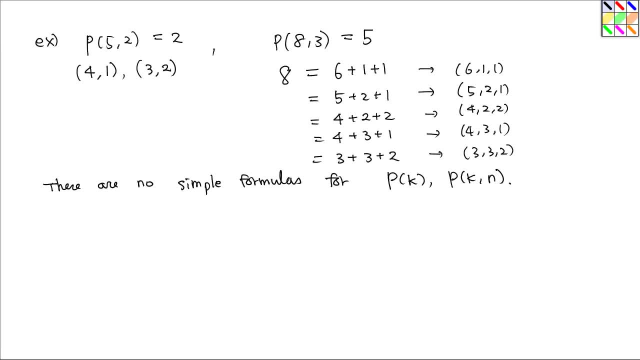 to compute this number And if you remember the 20-fold way we had this entry Number of ways to distribute k, I put identical balls into n identical boxes. So let me consider this condition without empty boxes. So it's like a surjective way without empty boxes. 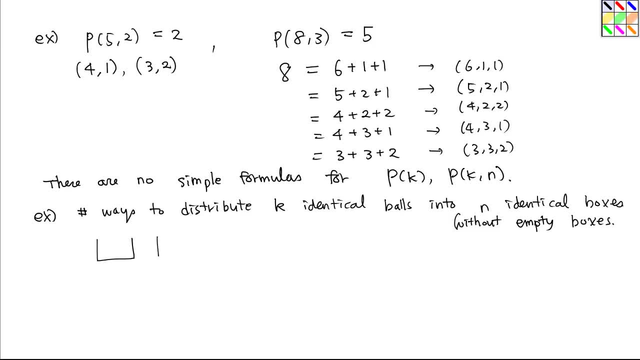 So, for instance, suppose we have four identical boxes and balls and are located like this, Something like this: And here what really matters is the number of balls in each box, and the order of the boxes are irrelevant, because the boxes are identical. So let me 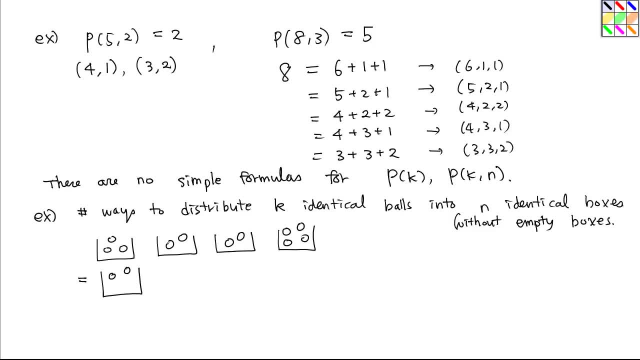 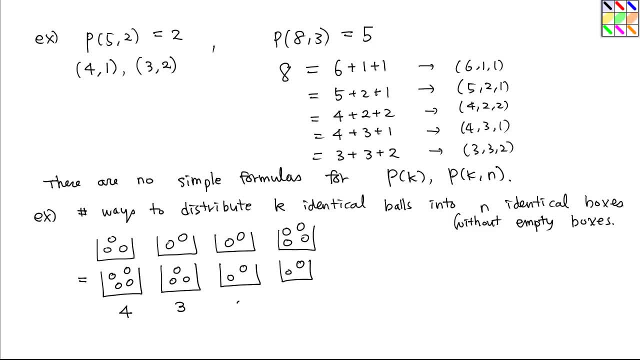 here is the number of balls in each box. So if you write this as a sequence, it's a decreasing sequence. It's going to be a partition of, in this case, k, And with this, the number of box. in this box should be size 4.. 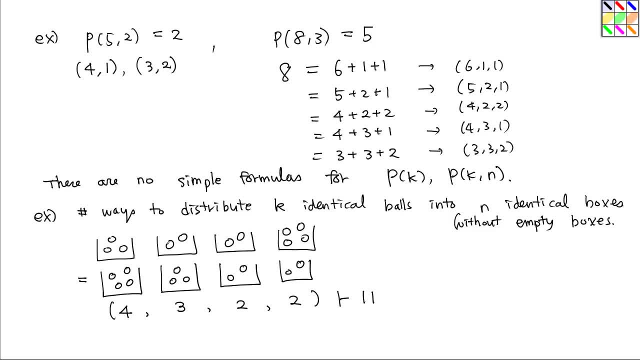 So show the number of boxes. In this case it's 11. 11. Eleven. So eleven is the number of balls And 4 is the length of this partition, or the number of parts of this partition is the number of boxes. 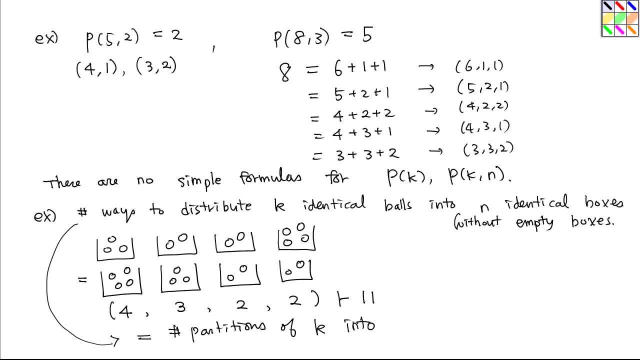 So this number here will be equal to number of partitions of k k-balls 3. into n parts. This can be written as p in our notation. Alright, so here we had this condition without empty boxes, but we can remove this condition. 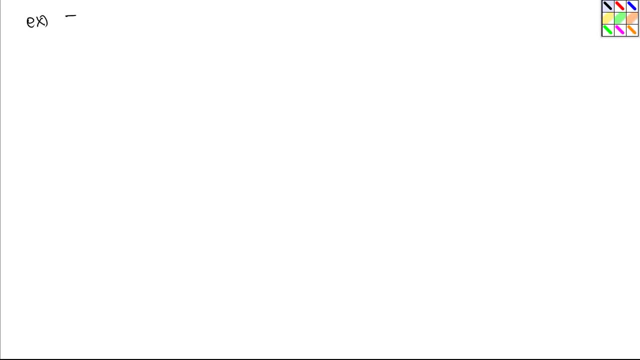 So number of ways to distribute k balls into n boxes. But some boxes we may have, some empty boxes. So if we distribute the balls then we can use only n boxes. So we can divide this situation into the number of. 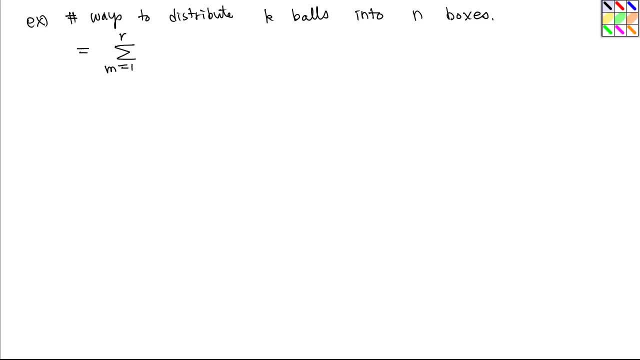 boxes used, So we can have at at most n boxes. So here is the same distribute number of ways to distribute k balls into n boxes. You can place your chooses here. you can place your choices here: boxes where only m boxes are used, meaning m boxes are non-empty and the remaining n. 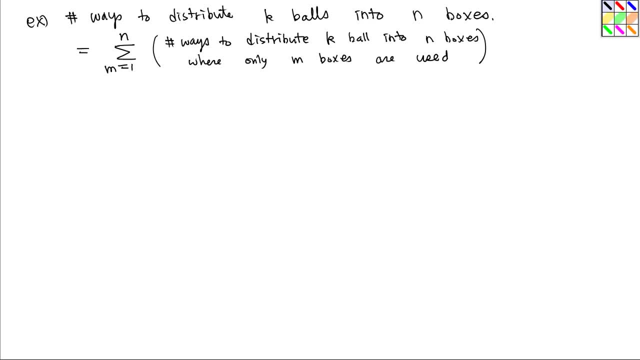 minus m boxes are empty. But because the boxes are identical, we don't have to choose m boxes in different way. There is only one way to choose m non-empty boxes, because boxes are all the same We have. so this here. we can just assume that there are only m boxes and those m boxes. 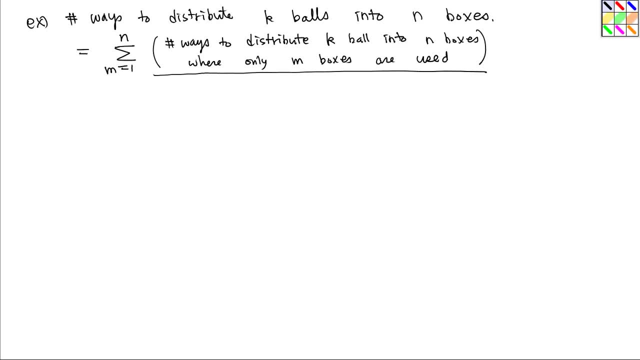 are non-empty, And in the previous example we found that this is equal to p. So if I write this again, sum m goes from 1 to n p. So this is the answer to this question. Okay, All right. 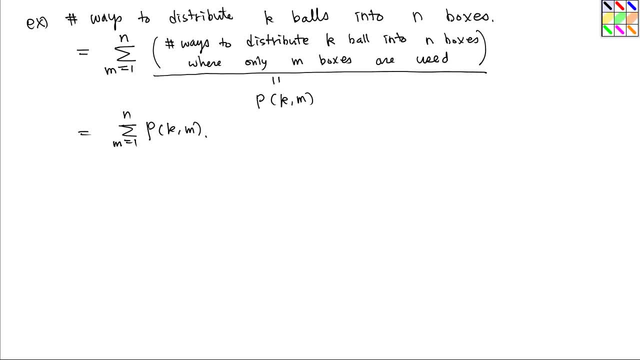 We can also consider partitions with some more restriction. We say that a partition, say lambda, lambda 1, lambda l, has distinct parts If the parts are distinct, literally so lambda 1 less than lambda 2, less than no equality. 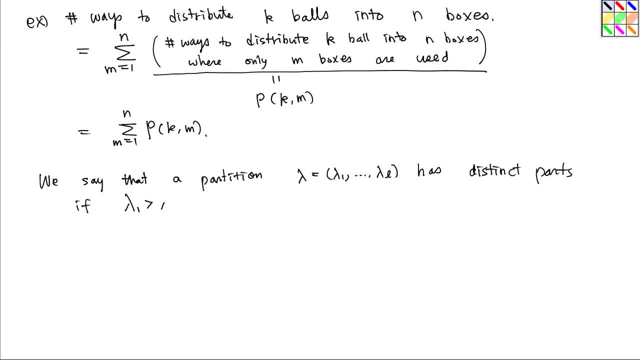 So that is, all parts are distinct, No parts are repeated. So, And we denote the number of parts. Okay, Okay, We denote the number of partitions of k into distinct parts like this: So q is the number of partitions of k into n distinct parts, n parts, and they are all. 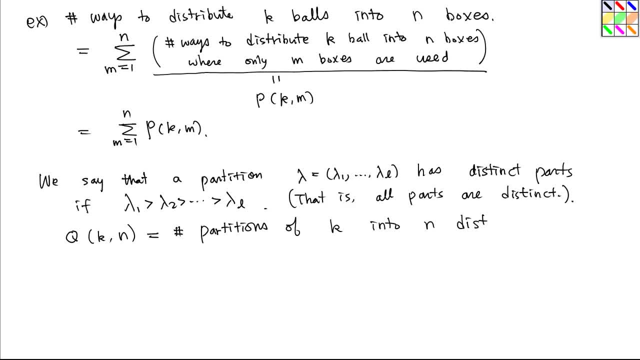 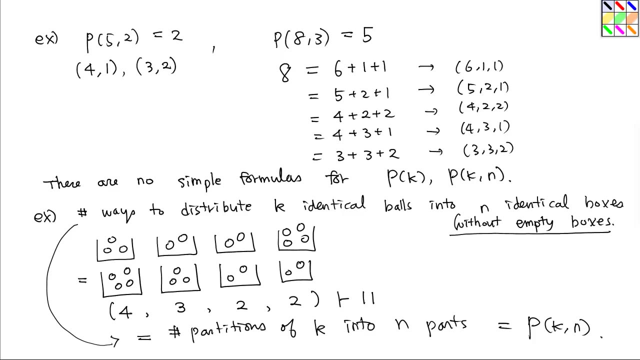 distinct. So for instance q- Okay of 3 comma, 8 comma 3 is. let me go back to this. so here, if you look at each partition, this one it has repetition, so we don't want this. this one is: every number is distinct, so it's okay. this part 2 appears twice, so it's not. 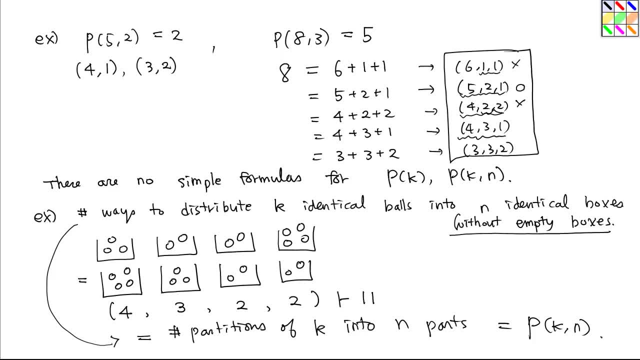 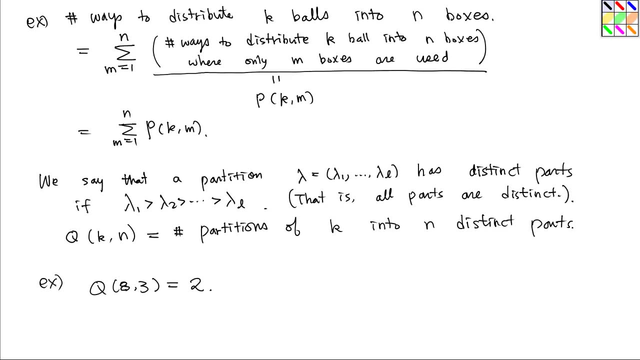 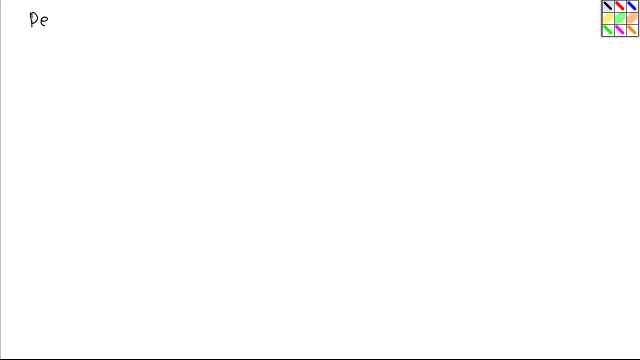 distinct partition. every number is different, so is it okay? this one, 3, appears twice. no, so there are two partitions with distinct parts, so this will be 2. okay, and there is a very nice way to represent the partition: graphical way, so let lambda be a partition, lambda 1. 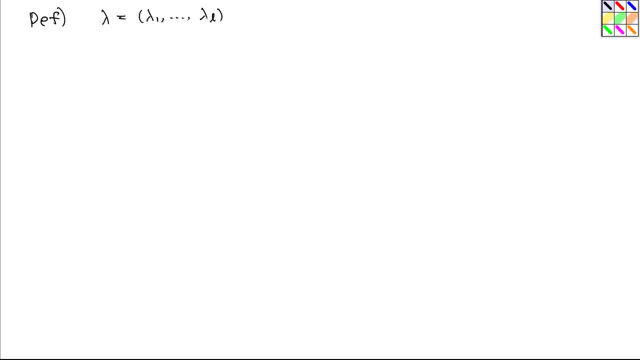 dot, dot dot. lambda L partition and the Ferris diagram. there is diagram, or also called young diagram, of lambda is just diagram, without diagram problems. and there are. didn't try to learn the second drawing. it stays the same, even though it is more flat. okay, let's makeYes. okay, so to. 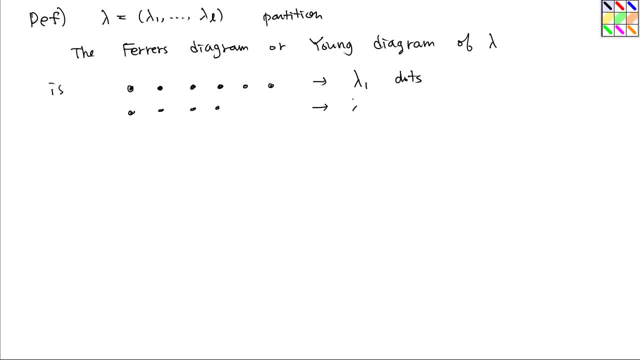 represent lambda 1 and to represent it we need I this. so right there, we have lambda on this one, we need x and then lambda down here. what about we put lambda l dots. so in the first row we have L 1 dot, in the second row we have, and then the last. 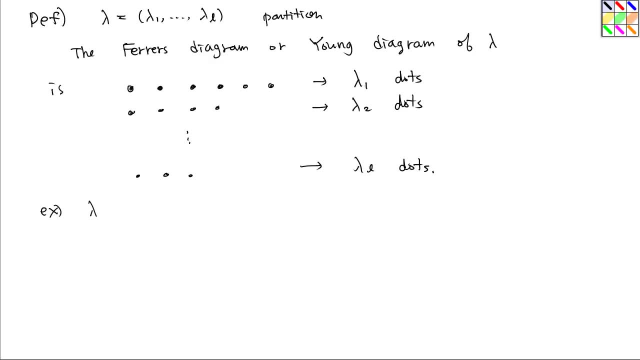 explain this using example. so lambda equals say five, three, three, two. then we draw dots, five dots in the first row and three dots in the second row, three dots in the third row, two dots in the third row, like this, and we always arrange the to the, the. the array should be left justified, meaning that they are all. 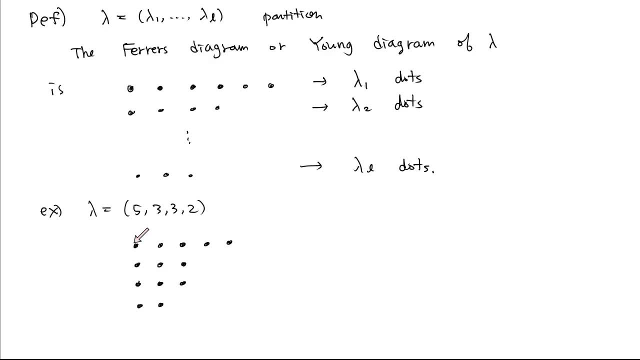 aligned in the left, leftmost dots and also it's. it's also common to use boxes also. we can use boxes. I mean so, for instance. I mean so, for instance. I mean so, for instance, draw five boxes: one, two, three, four, five and three boxes, like this. so I'm just